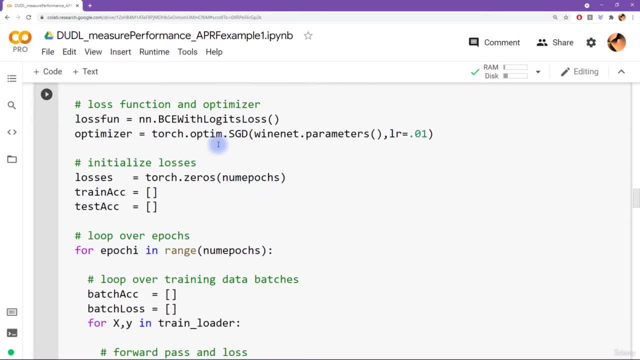 Not a whole lot of stuff going on in here. That's really interesting. We've actually discussed previously in the course that you know, stochastic gradient descent is not necessarily the best method, The best optimizer for these data. We can do a little bit better. 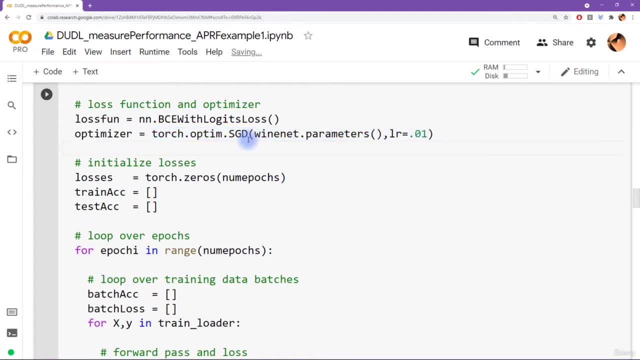 But, as I've also mentioned before, there are plenty of cases when studying deep learning where you actually want to make the model do a little bit worse. You want to drag down the performance a little bit, to increase the variability in the performance, which is going to facilitate a discussion and understanding of these different performance metrics. 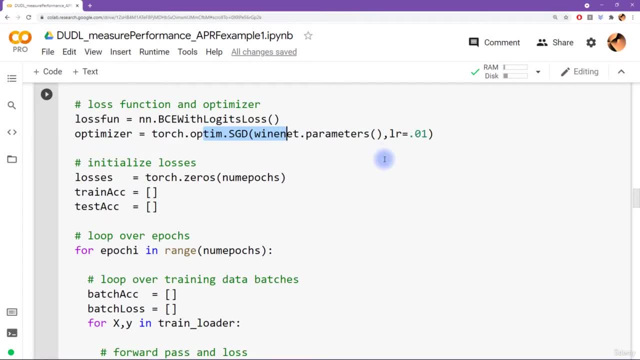 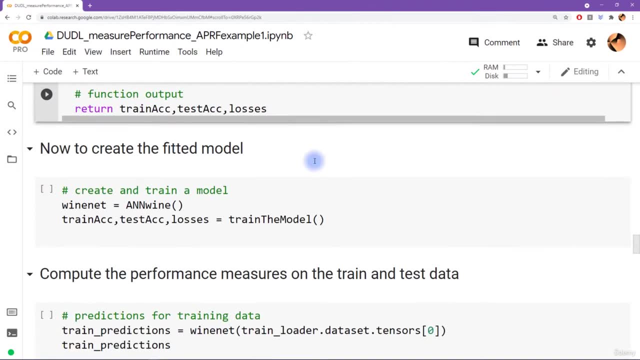 In particular the difference between recall and precision. Okay, anyway, the rest of this code is pretty straightforward stuff you've seen now many times. Okay, so here we train the model, We get a new model instance and then we train the model. 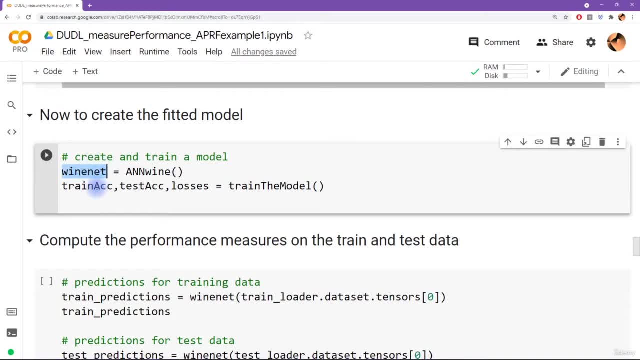 So now we have our model instance, which is fully trained, So it has trained weights, and we have these metrics. But in fact we don't really care about these for this particular video, because we are going to compute the new performance metrics. Okay, 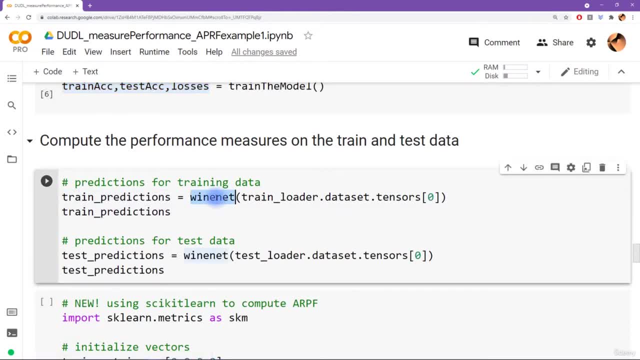 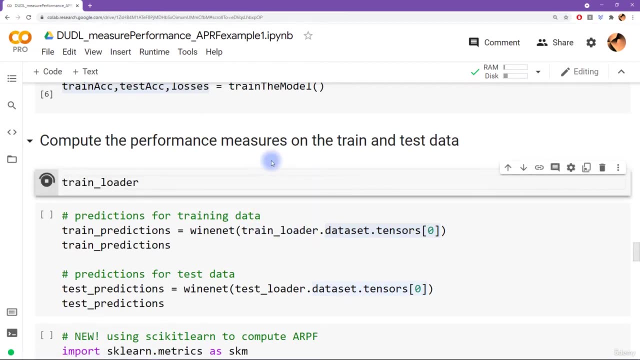 Down here. So what I do here is take our model instance with the trained weights and everything, and input: train underscore, loader, dot, data set, dot tensors. Let me actually make sure we're all on the same page here. So the train loader is this iterable, is a type of data loader. 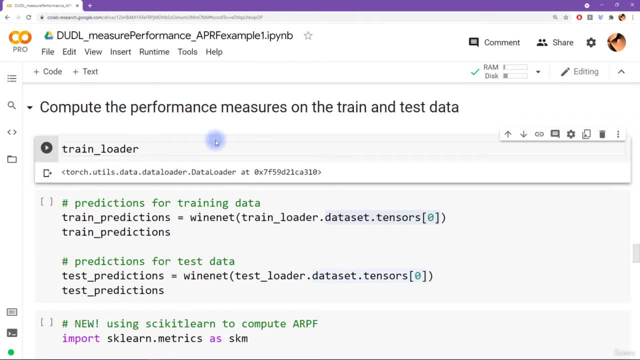 And normally we use this as an iterable in a for loop, But we can also access all of the data directly. So we say dot data Set and then this has dot tensors and we can see that this is a tuple of two pieces of information. 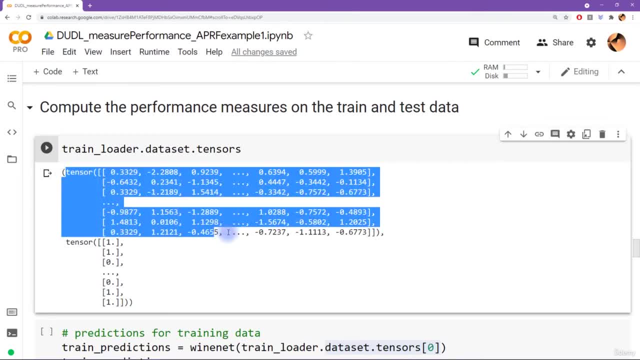 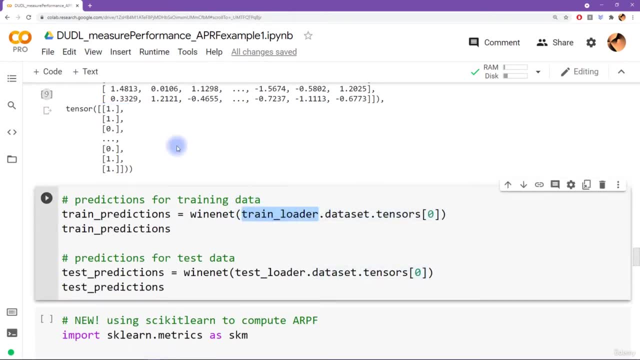 There's two items inside this tuple. The first one is all the actual data And the second one is the labels. So what I am doing here is grabbing all of the data. This is not just one mini batch. This is the entire data set. 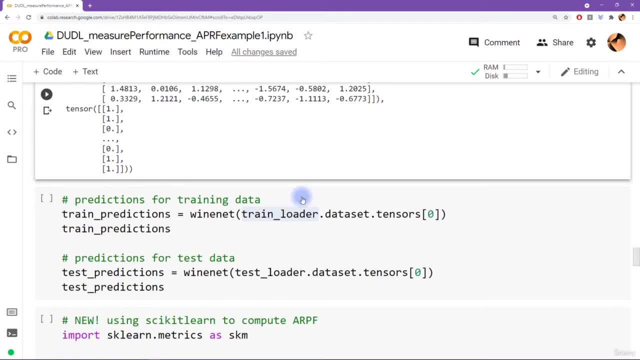 It's stored here as one big tensor. Okay, So I get all of the data, the training data, And Input that into the model and then get out the predictions. Let's see what those train predictions look like. You can see that is a vector of numbers. 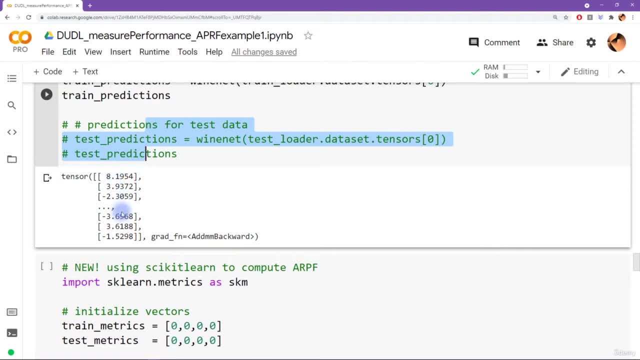 Now, these numbers are the raw outputs from the deep learning model from the output layer. This is not the output pass through a sigmoid function or a softmax function. The reason why that's important is that the predictions here are just based on positive or negative numbers. 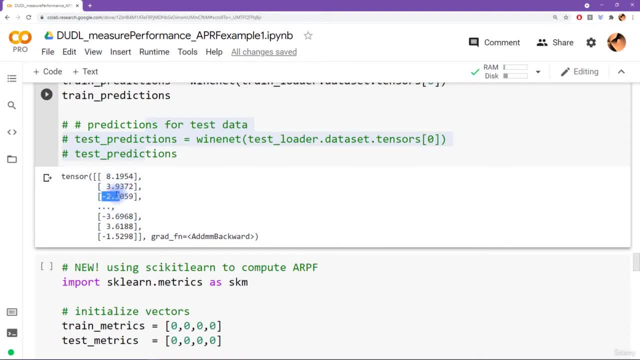 Basically the sign Of the number not based on 0.5.. So 0.5 as a threshold cutoff would be if these data were passed through a sigmoid function. Okay, So that's just a reminder for later. Of course, you know that already. 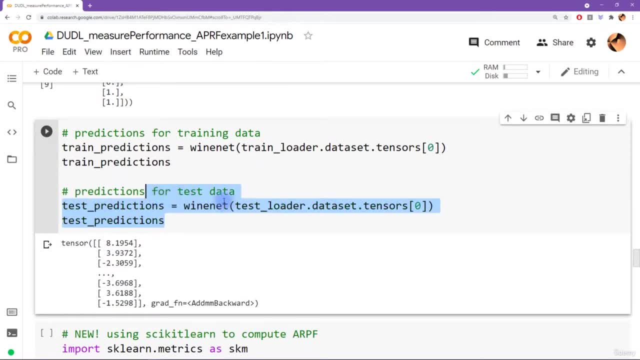 Here this code, here these three lines of code. we have exactly the same as up here, except we are inputting the test data instead of the train data. And here too, you know, it's also just to show you a little bit of variety. 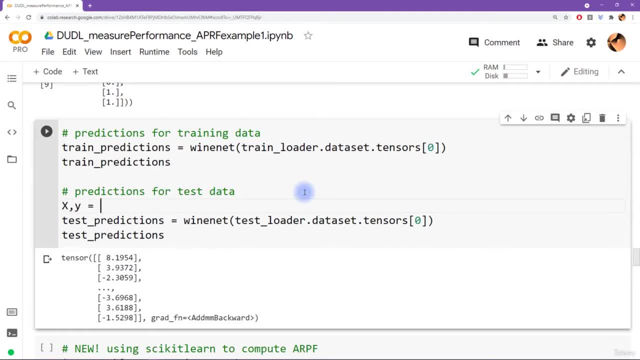 Because often in this course I do something like this: x comma y equals next iter test test loader like this: and then here x is going to be the same thing as this in here. Now these are the same thing because the test loader only has one mini batch. 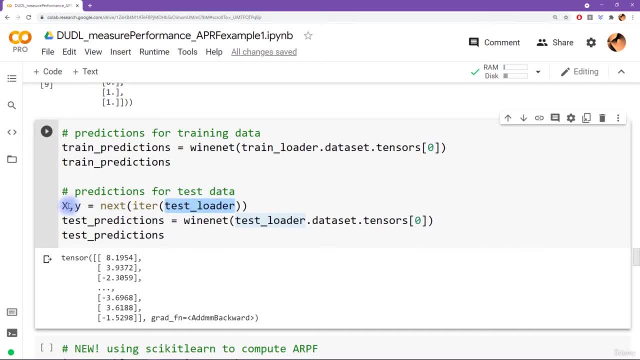 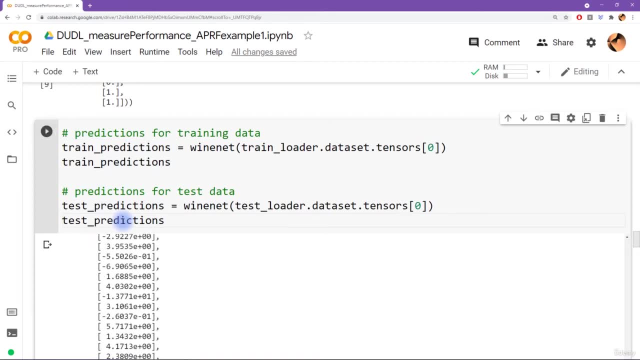 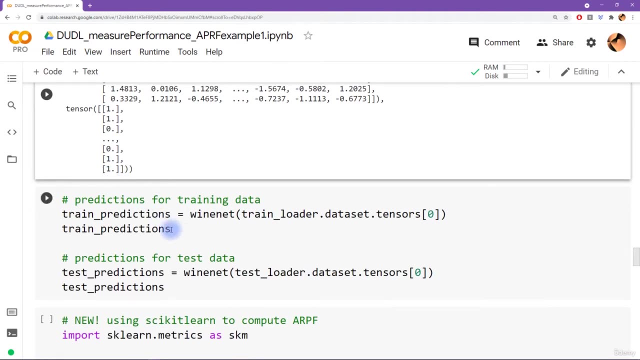 If there were multiple mini batches in the test loader, then in fact this would only be the first mini batch. So yeah, so then we get the predictions for the test samples. So now we know the target values. so the true answers here and we know the predictions here. 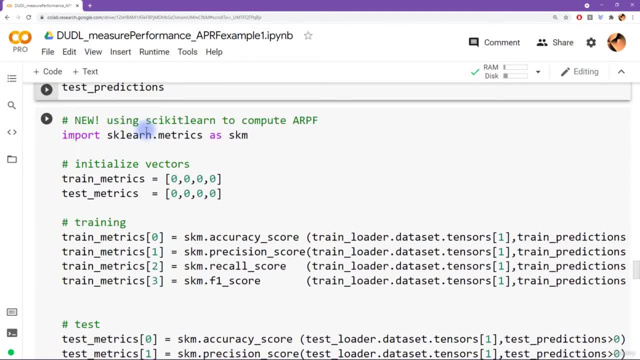 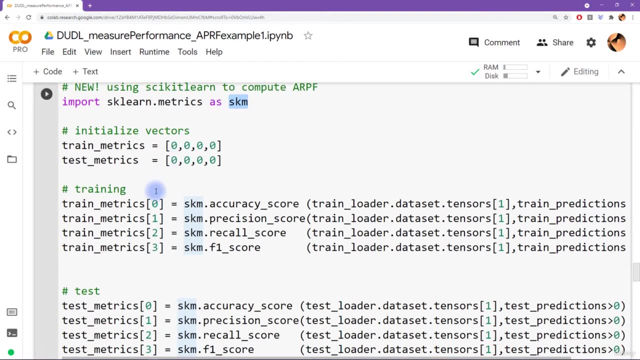 And that is what we input into this series of functions here through scikit-learn. So it's scikit-learnmetrics and we're going to import that using the abbreviation skm. So scikit-learnmetrics. And then here: 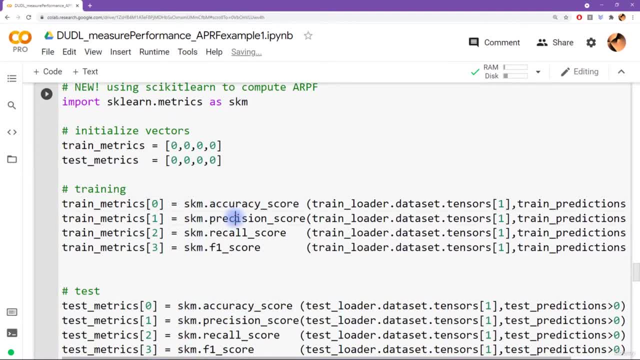 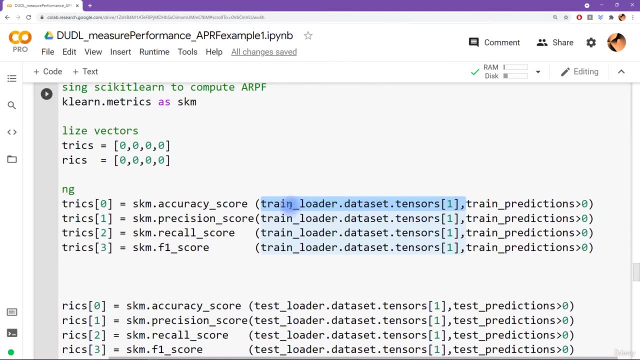 You can see I'm computing these metrics- accuracy, precision, recall and F1 score- And what we input here. we provide two inputs to this function And those inputs are the target values, right? So this is from the train loader. 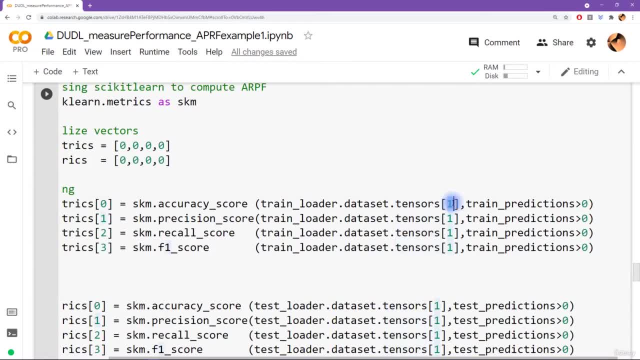 We have the data set and then the tensors, And then this is the second element of that tuple which I just explained a moment ago. So these are the target values. This is the true state of the world, The objective, The objective reality. 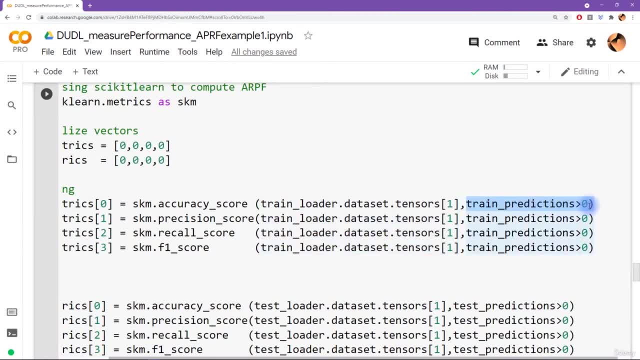 And then we have the model predictions, which is the predictions or the subjective reality. And here is you know. this is why I kept mentioning that we're getting the raw output from the model, Because if these were soft maxified or passed through a sigmoid, 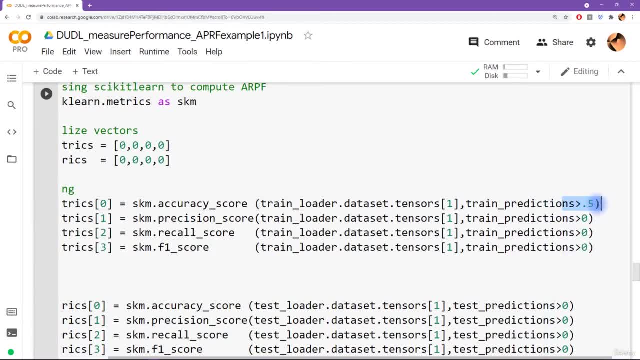 then we would actually need to specify this as 0.5 instead of 0.. Okay, so these are 0.. So this ends up being a vector of a Boolean vector of trues and falses, And this is 0s and 1s. 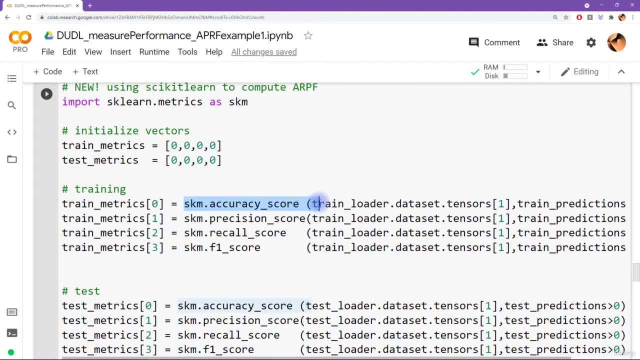 And then we let scikit-learn do all the like super duper, intensely difficult math, Totally kidding. The math here is really, really simple. We could actually just compute it writing our own code, like what you saw in the previous video. 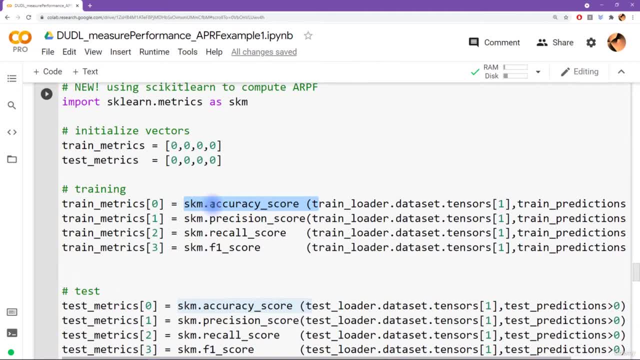 But many people often do this through scikit-learn, So I wanted you to know how to do this in scikit-learn. Anyway, here are our four metrics for the training data And here are our four metrics for the test data. 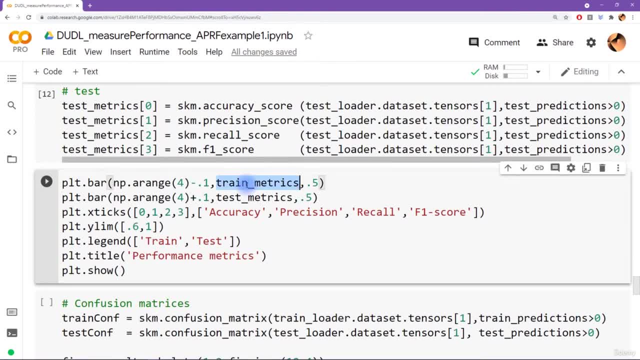 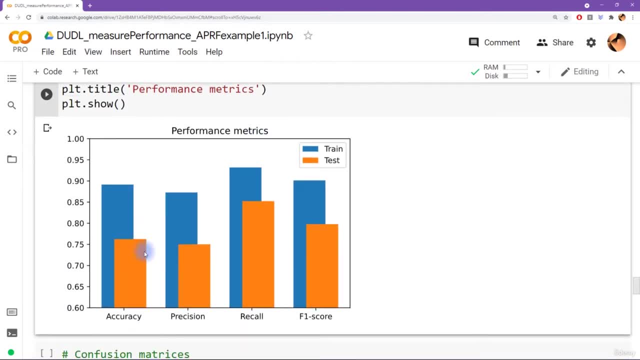 And now I'm going to create a bar plot that shows the train metrics and the test metrics in the same bar plot. Now, this one is accuracy. So this bar here actually corresponds to what you would see at the very end of how we normally visualize accuracy, as you know, as a function of training. 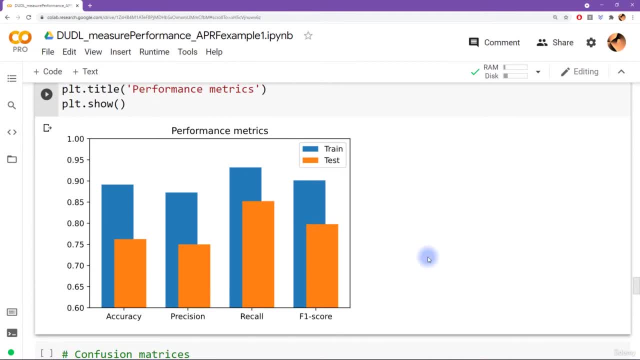 So normally you see this like logarithmic type function going up And then And then the very last point. so the final training epoch would be what these two numbers correspond to. So this gives us the accuracy for train, almost 90%, and for test, where it's about 76%. 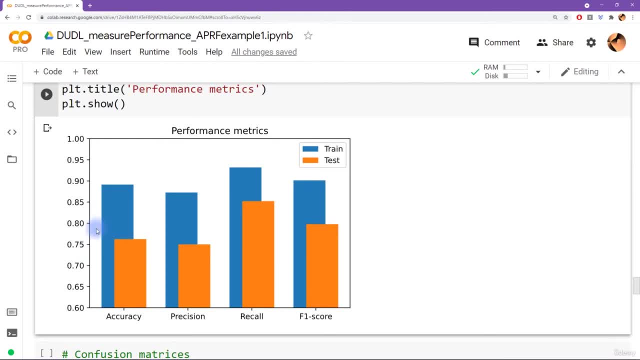 So not super great. I think you know we could work on this architecture and get this higher a bit, But we don't need to worry about that for now. So then it's interesting to see that the precision and recall are actually not the same. 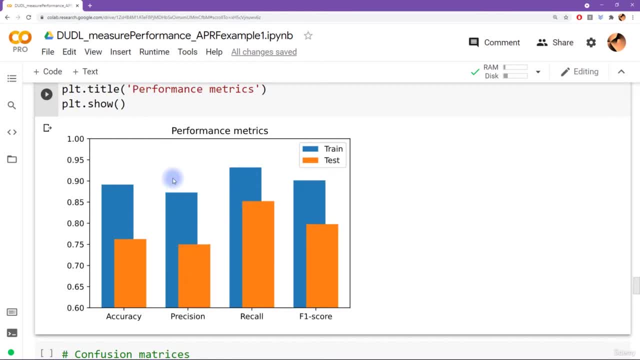 So the recall is a bit higher And the precision is a bit lower, And that's true for train and also for test, although it's more apparent in test in this case. So what does this mean? How do we interpret this? Well, remember that recall and precision are both telling us about the model biases. 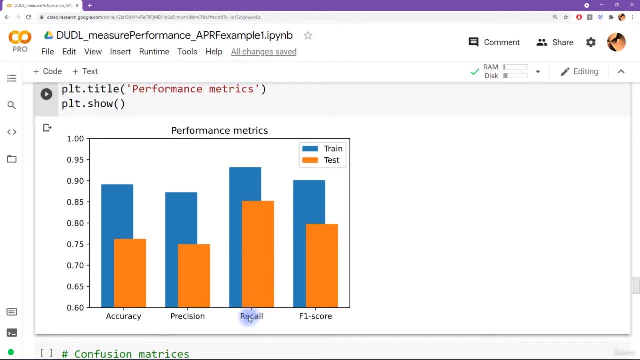 Recall is that the model has a bias for saying no, which in this case, in these data, this means the model has a bias for predicting low quality wine, And precision would mean that the model has a bias for predicting low quality wine, And precision would mean a bias towards saying yes, which in this case, means the model has a bias towards predicting a high quality wine. 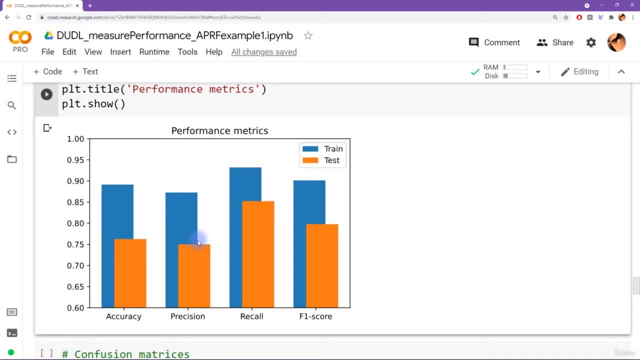 So the fact that the recall values here are higher than the precision values tells us that the model actually has a bit of a problem with saying yes too often. So the model is rating too many wines as being high quality. This model would actually make a great sommelier right. 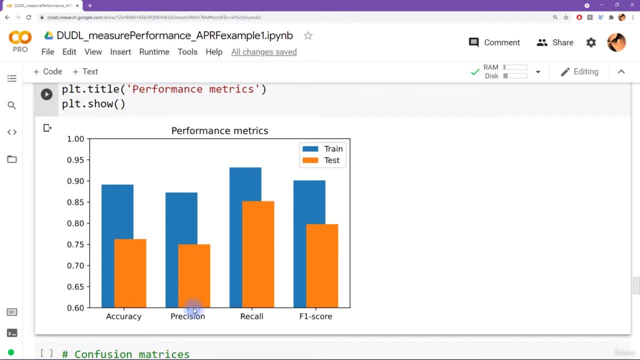 This is what you want in a sommelier. It's better for a wine expert To you know, as someone at a restaurant trying to sell you wine. it's better for them to say that all these wines are great than to be biased where it's saying that all these wines are terrible. 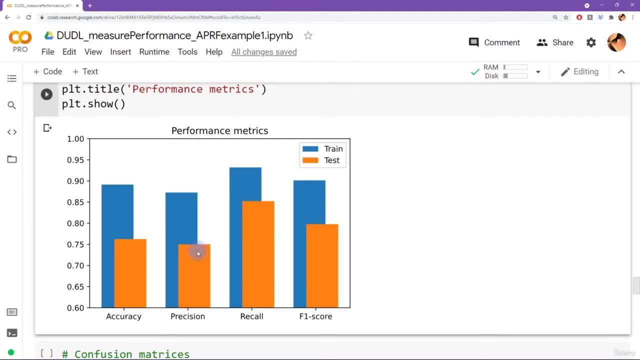 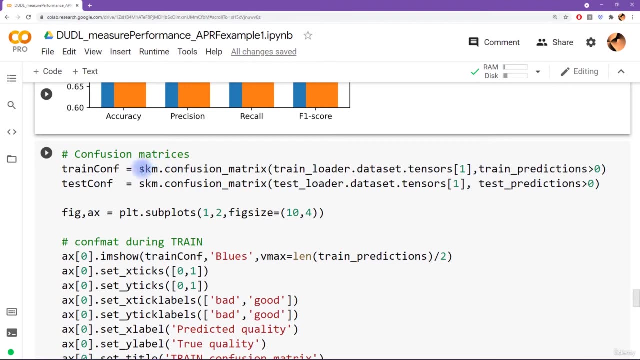 Okay, And then here you see the F1 score which, as I mentioned before, is kind of. it's not literally an average, but it's basically a mixture between precision and recall, So it's somewhere in between. Okay, So these are the bar plots, and now we can visualize this in a confusion matrix. 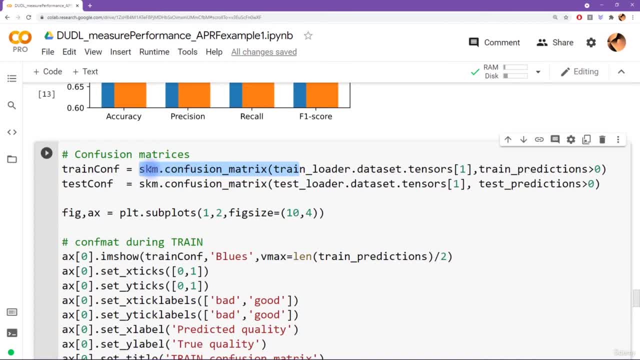 So this is also something that You can do with the Cykit-Learn dot metrics library. So same concept. we input the target values and the actual values, So the true state of the world and the predicted state of the world from the model. 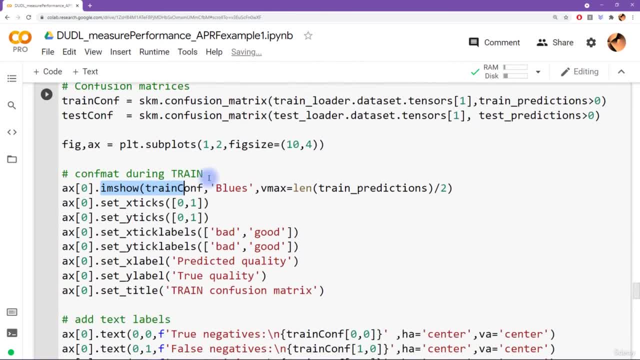 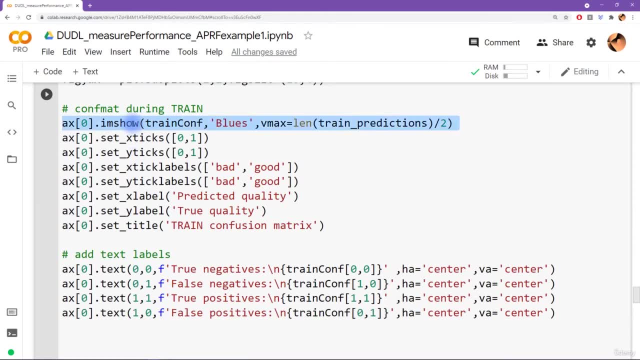 And then we can visualize this confusion matrix as an image. And well, there's a lot of code in here, but it's mostly, you know, this is the most important line here. This visualizes the uh matrix. This is just, you know, making the 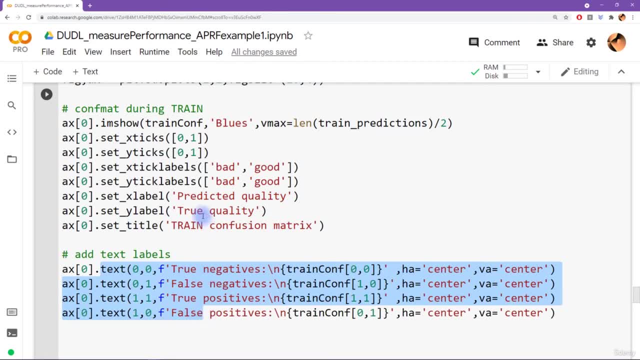 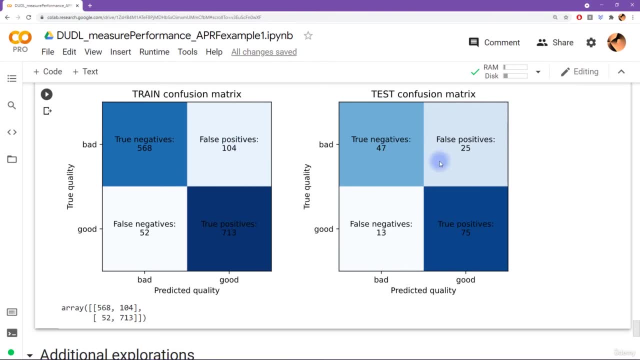 Figure look a little bit nicer. And then here I'm adding the text labels on top. So, and then repeat for test. So here we see what that those two matrices look like. Now you always expect that in these confusion matrices the diagonals are high. 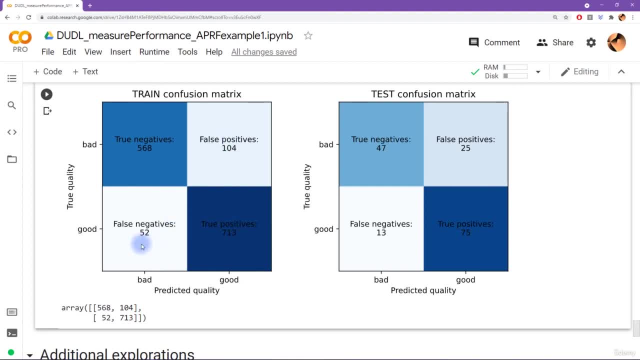 These are the correct answers, and the off diagonals are relatively low. Now, ideally, these off diagonals should be really low. They should be very close to zero, which they are not, but that's okay. But, uh, but Certainly the diagonals should be larger than the off diagonals. 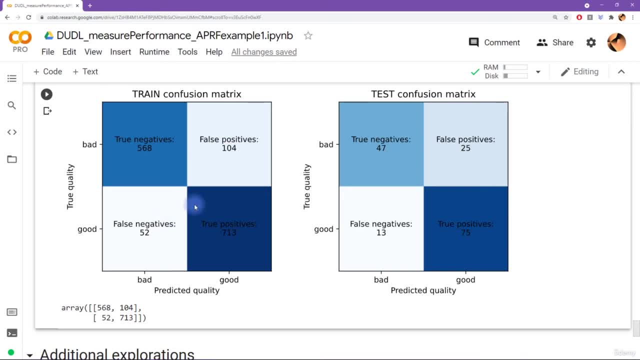 Now another slightly annoying thing, or maybe a little bit more than slightly annoying, but a confusing thing about these confusion matrices in Python and scikit-learn is that they swap the columns and the rows. compared to what how these things are often visualized. 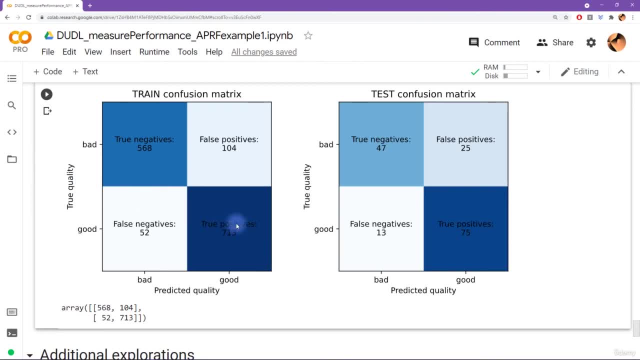 So here we have the true positives in the lower right, Whereas what I showed in the slides was the true positives on the top Left And the true negatives were on the bottom right. There's a additional exploration here, that's asking you to explore that and and correct for that. 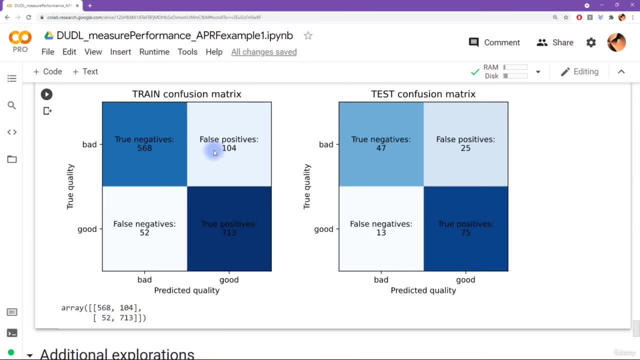 Okay, But it's also interesting to see that the number of false positives is higher and the number compared to the number of false negatives. We see that during training and we see that during a test. In fact it's it's pretty much exactly double the number of false positives compared to the number of false negatives. 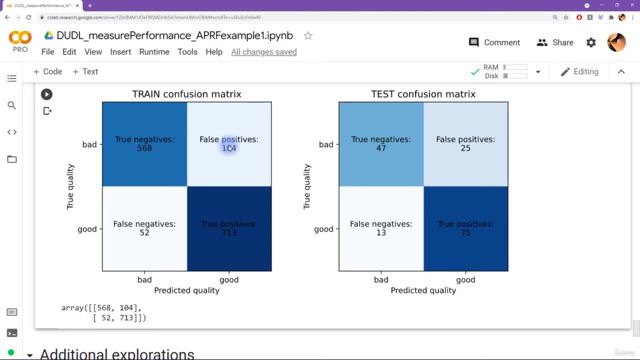 So what does that mean? Well, that means that our model has a bit of a bias towards saying that the wine is good, And that is why the precision is relatively low compared to the recall, which is a little bit higher. So those values that we interpreted with the bar plots are here represented in this confusion matrix. 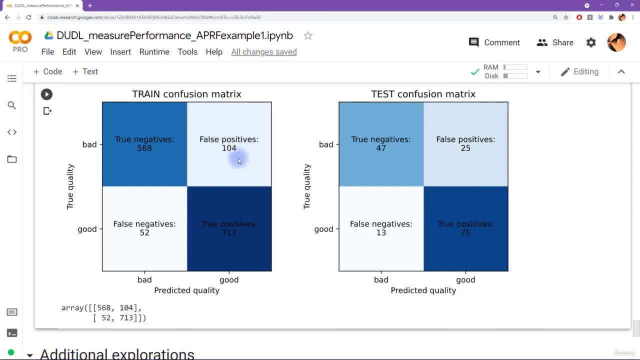 So, again, the model has a bit of a bias towards giving false positives. So the model is biased towards saying that wines are good, High quality wines, when they're actually not. they were actually rated as being relatively bad quality wines, or, at least you know, lower quality wines. 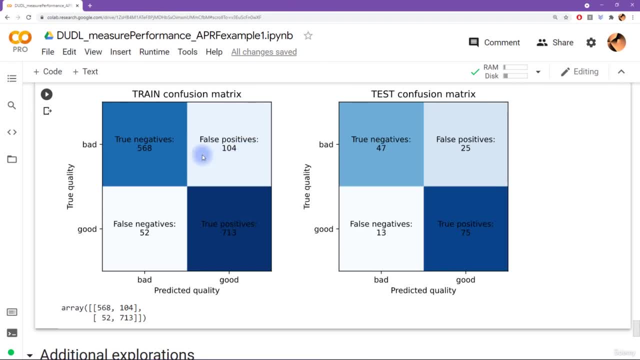 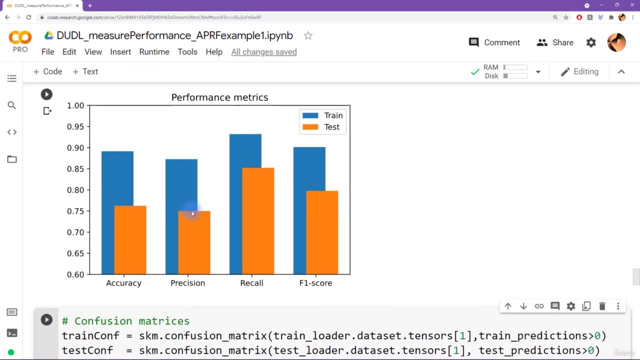 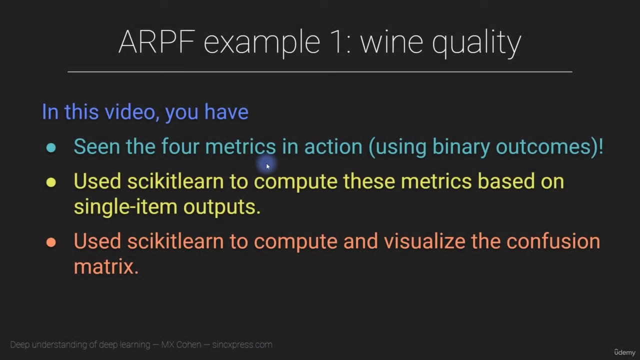 So we have a bit of a bias here. So this means that the precision is going to be lower than the recall, And that is what we also see up here. So the precision is lower, Recall is relatively higher. So that is the different signal detection theory. derived metrics. 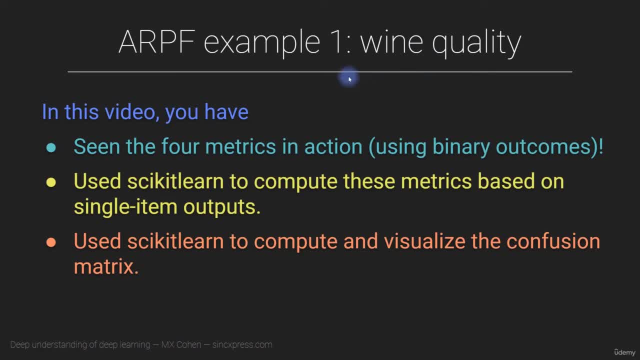 In the wine quality data set. stay tuned for the next video we are going to repeat conceptually similar but with the endless data set, we're going to have to learn a couple of new tricks for dealing with multi class categorization.